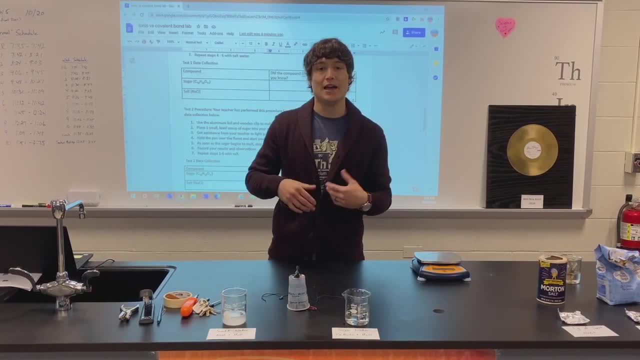 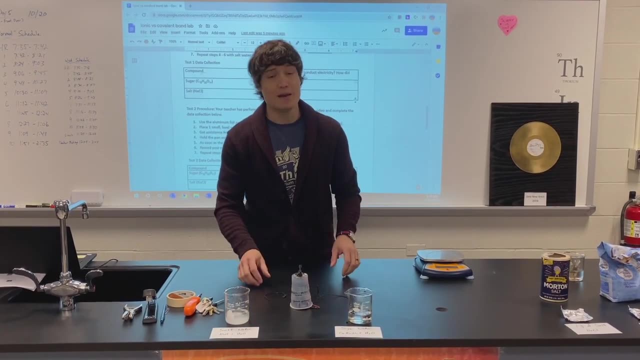 will actually bounce from one atom to the next, And that's what electricity basically is. So what I made was a little conduct-o-meter 3000 patent pending on that one. So what I walled is really is just a circuit. So I have a battery. 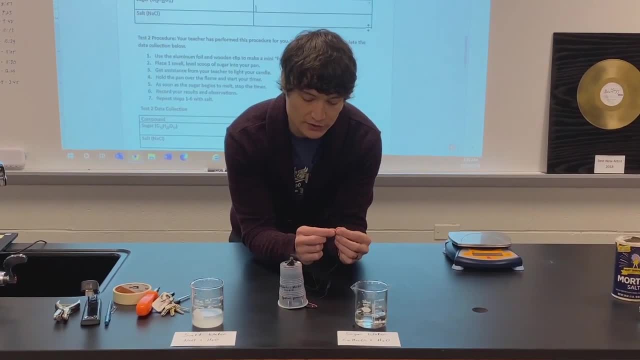 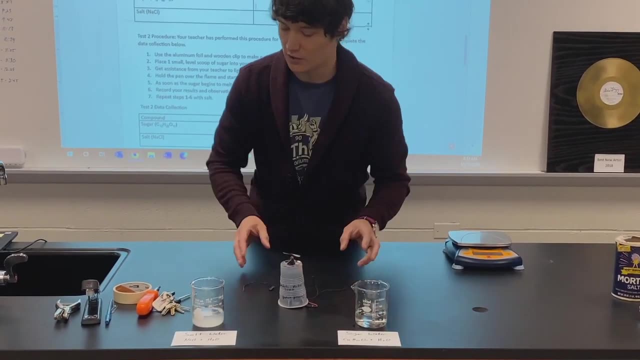 pack hooked up to this little propeller. If I close the circuit, the propeller will spin. It's showing that the electricity is in fact conducting through the wires, making the motor spin and continuing the circuit. okay, We could just test some random objects. Screwdriver. 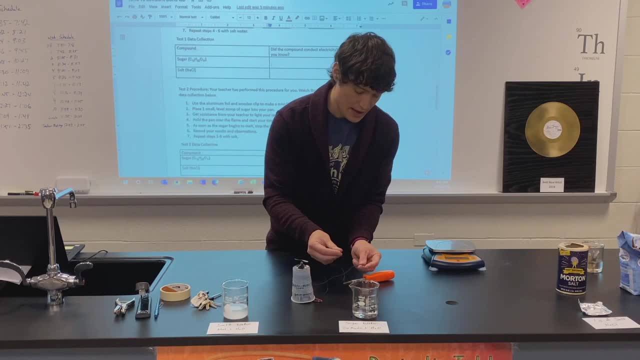 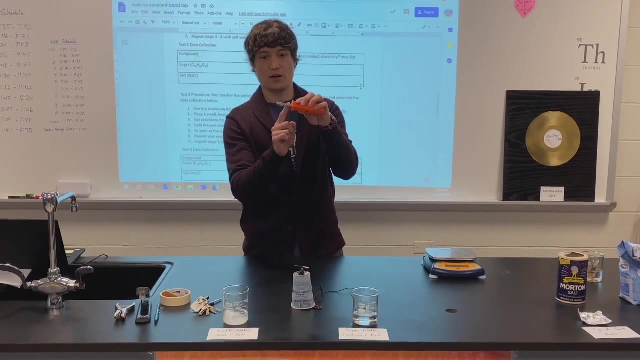 We'll take a look at the metal part of the screwdriver And you'll notice that the metal part of this. I'm not going to touch these, I'll just kind of put them on the screwdriver and it will make the propeller spin because the electricity is in fact running through. 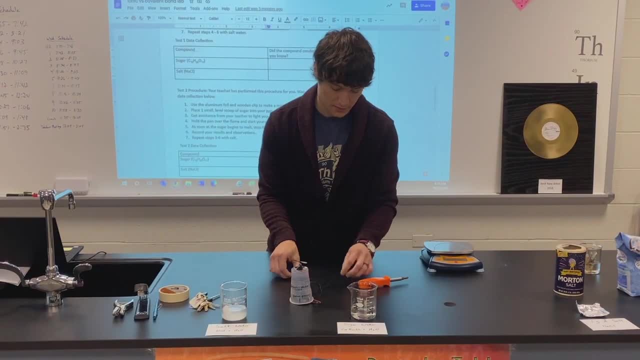 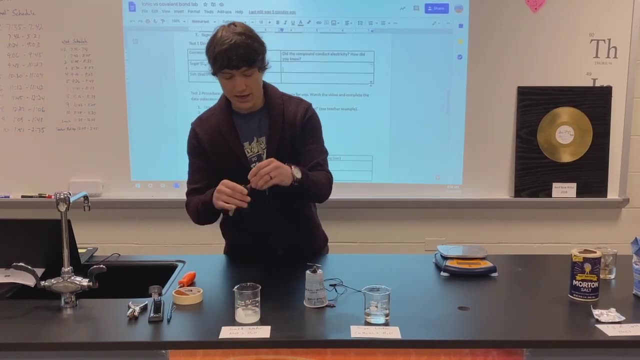 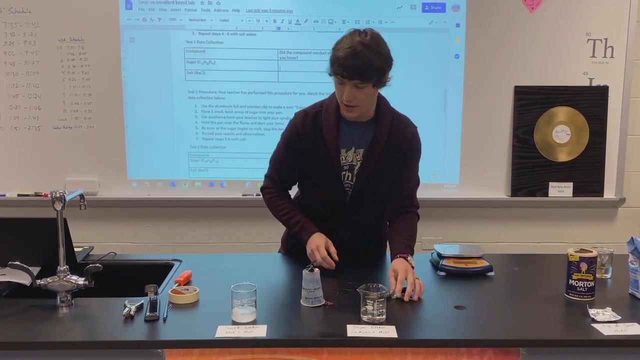 the screwdriver. If I try it on the handle of the screwdriver, which is plastic, no conduction there. all right, Key key to my car. Again, the metal part is going to conduct, The plastic part, not so much Hole puncher. make a prediction in your head right now. What do you think is? 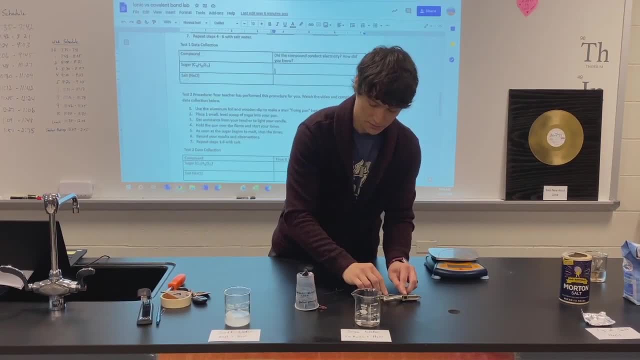 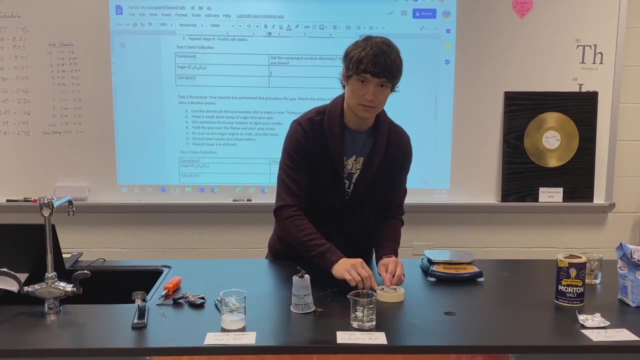 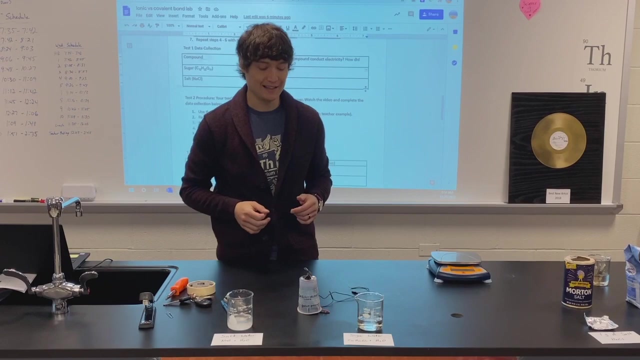 going to happen with the hole puncher Conducts Pen. Let's try the tape. We already did plastic Tape, Not so much, okay. So again, our different types of compounds. one will conduct, one will not. Let's test them out. So I'm going to put one end of the probe into the water. 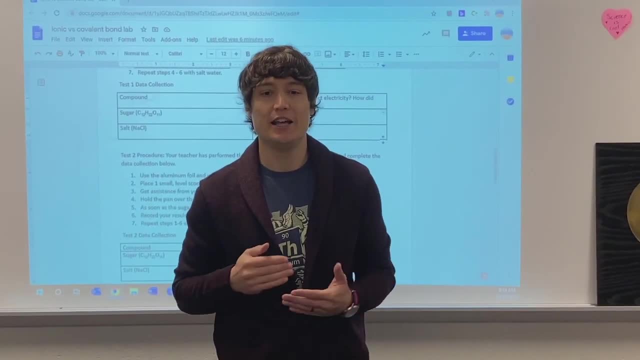 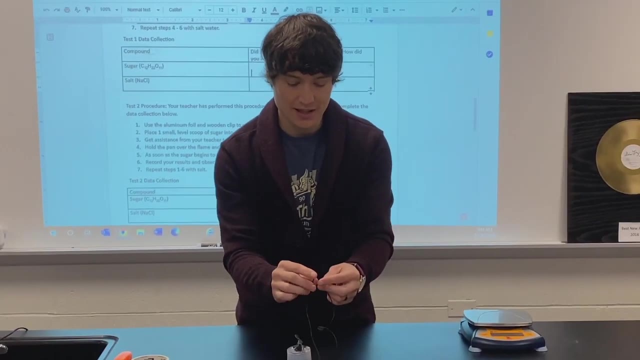 Now, normally, guys, disclaimer here: you are not going to introduce electricity to any liquids ever. okay, This is an extremely low current. I could even touch them. Nothing's going to happen because I'm only working off the AA battery here. okay, So there's not. 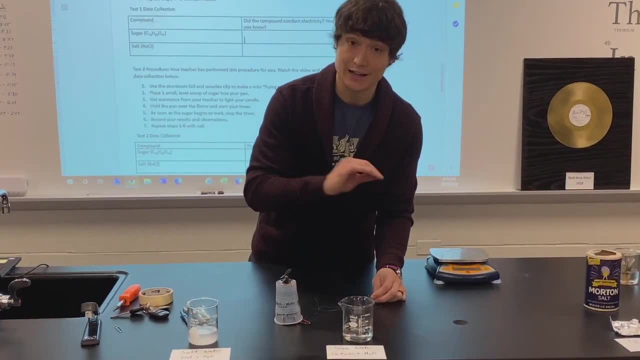 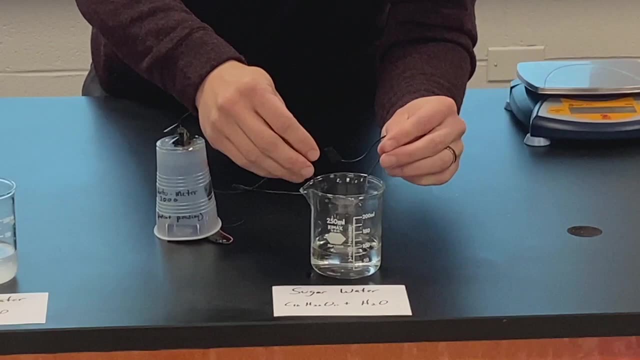 a whole lot of danger here, But normally you're never going to try something like this at home. So let's try the sugar water first. I'm going to put one probe in on one side of the beaker and the other probe in the other. I want to see if the electricity will actually. 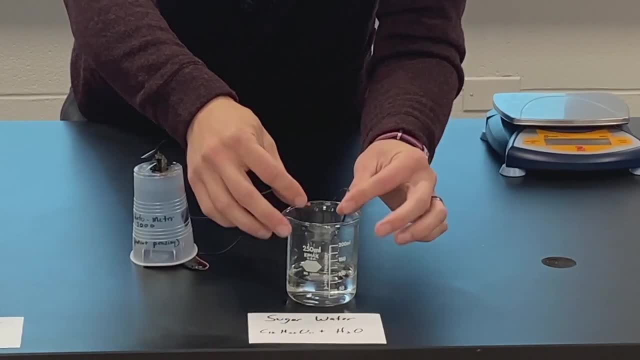 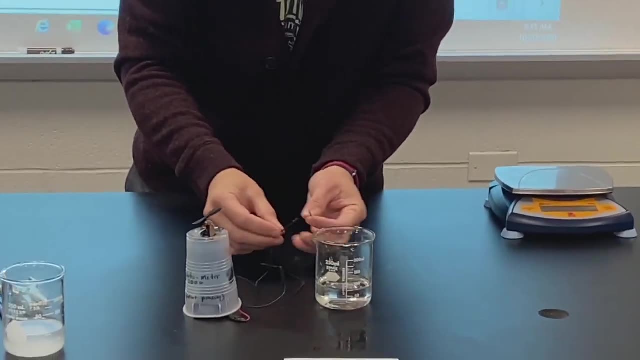 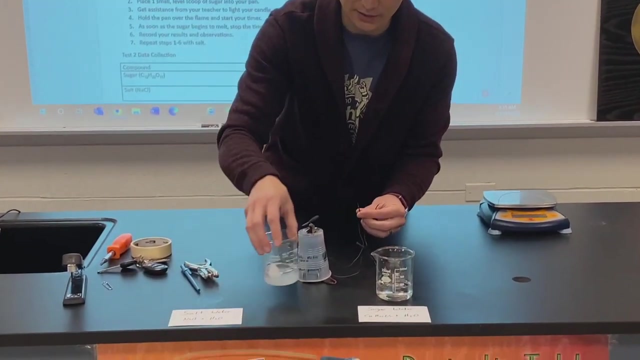 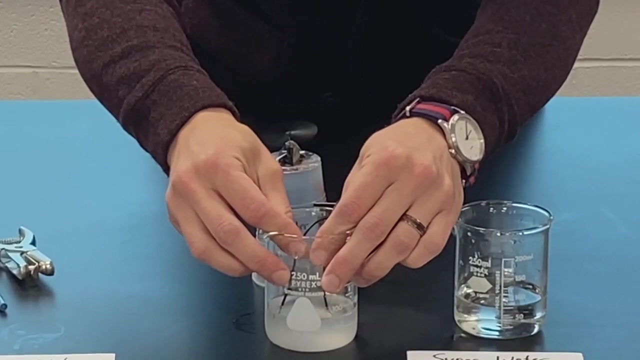 run through the liquid and meet the other probe And you'll know if the propeller spins. And I got nothing. Dry And let's try the salt water Again. I want you to notice the probes are not touching in the solution. The electrons are flowing through the solution. 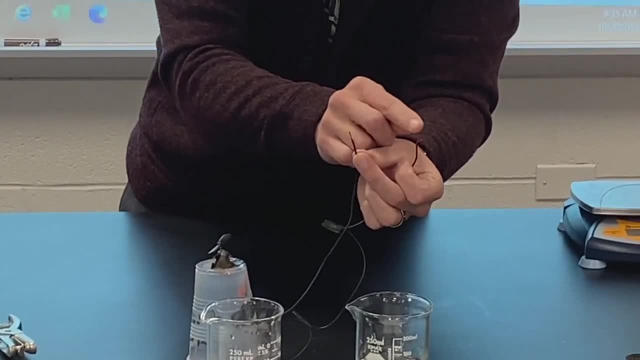 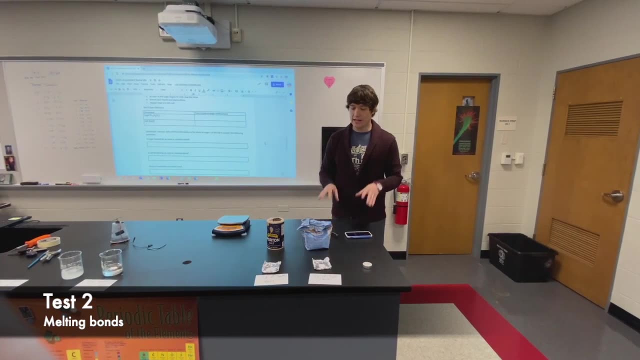 to close the circuit going through the water, to close my circuit. So that isn't factoring In fact conducting electricity. All right, guys. next up we're going to take a look at again an ionic and a covalent bond, a compound, to see which one will melt quicker. 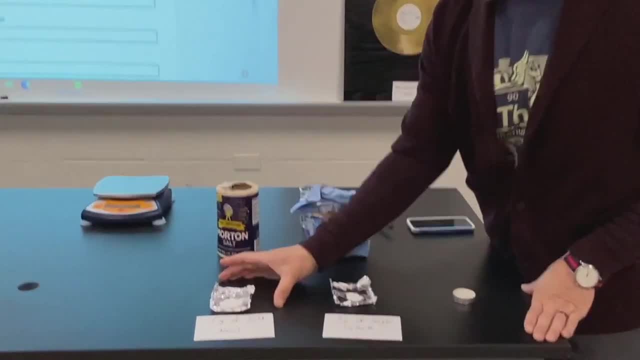 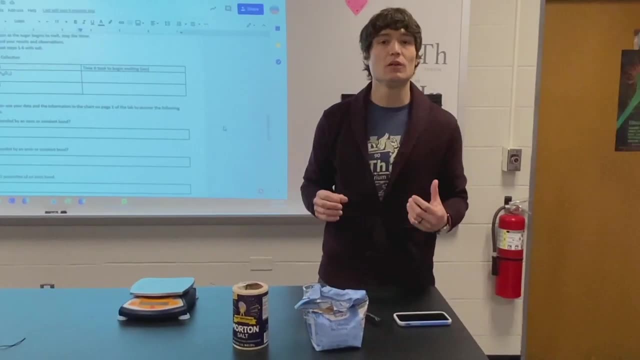 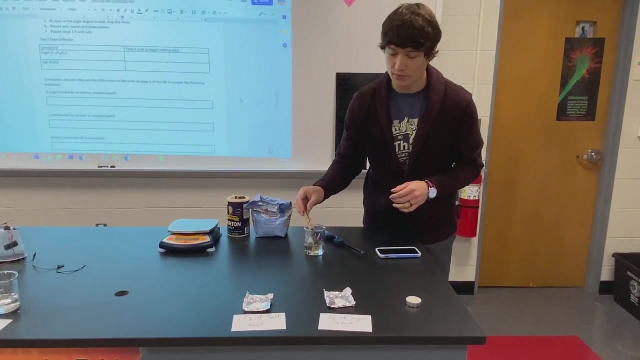 So I have just plain old salt and just plain old sugar. I measured out exactly one gram of each on my balance over here, And we want to see how long it takes for each of them to melt. So what we're going to have here is little homemade frying pans here for you. 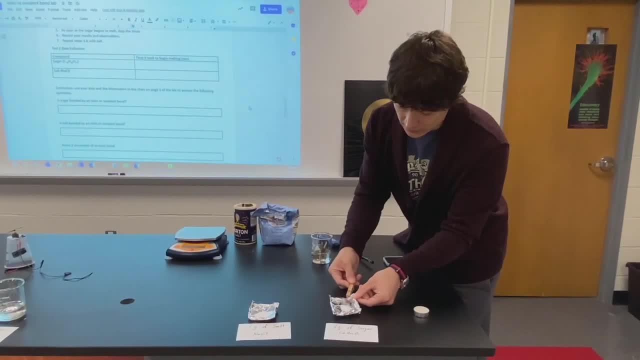 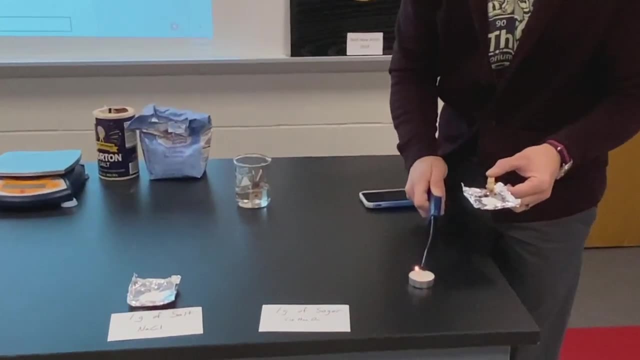 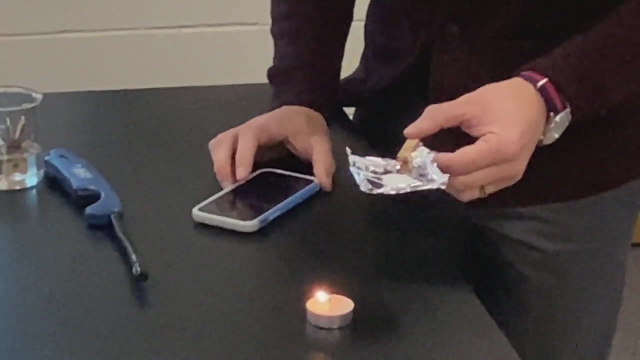 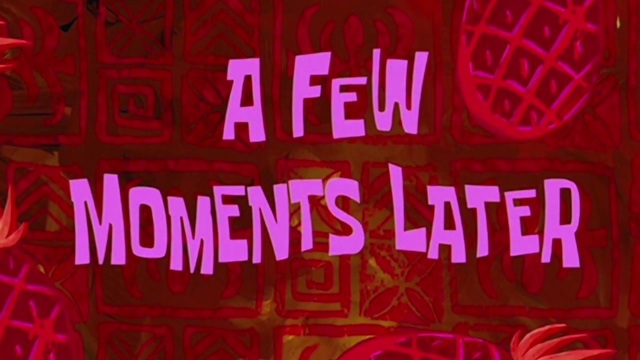 Soak them in water so they don't light on fire. Just going to pinch one on the end here, starting with sugar. This one is sugar Light, my key tent, my tea candle. I'm going to start my timer as I lower it down onto the flame. 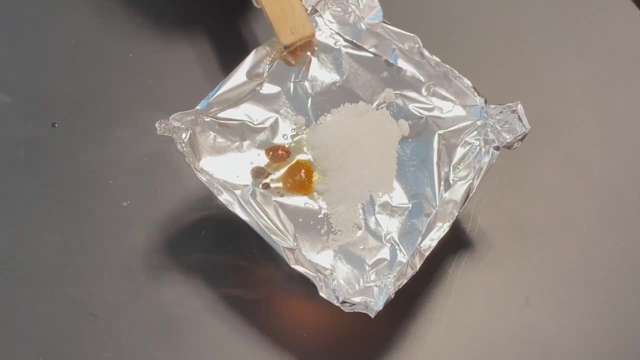 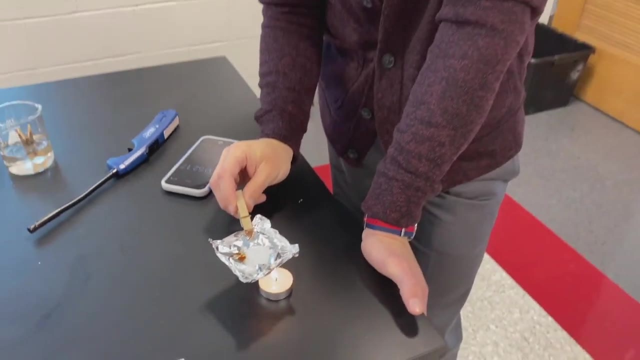 As you can see, my sugar is starting to melt. at about 45 seconds It began to melt. I'm not going to keep melting it because it's going to start to burn and smoke And I don't want to set off the fire alarms, So we're going to stop it at 45 seconds. 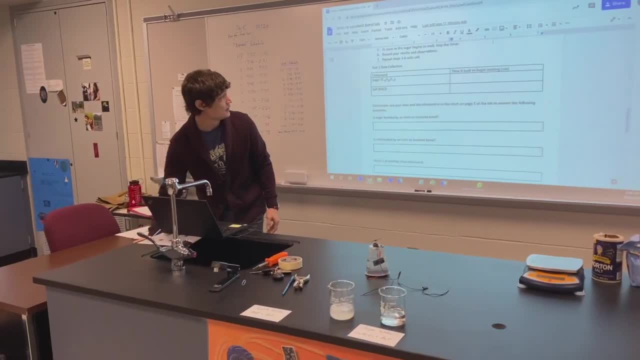 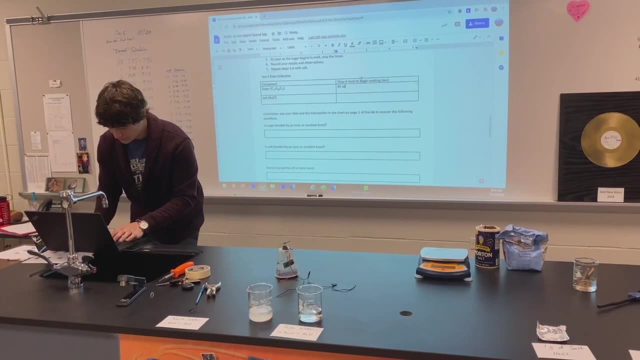 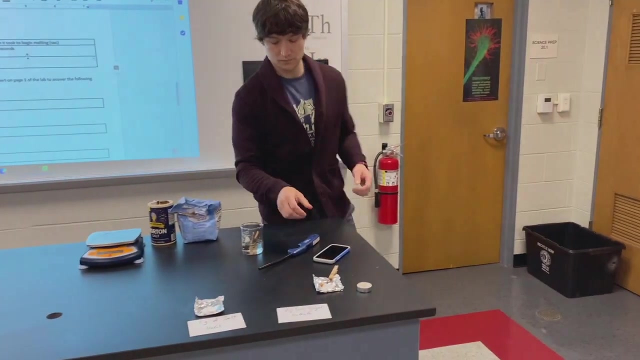 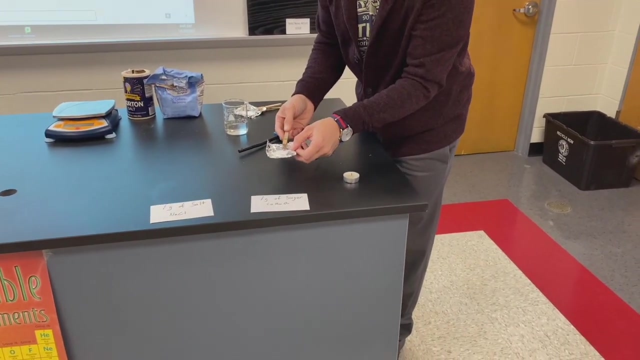 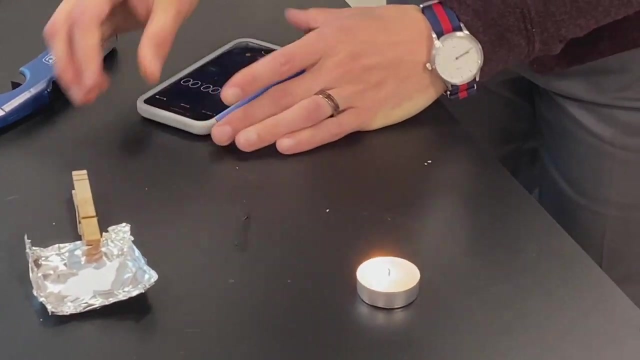 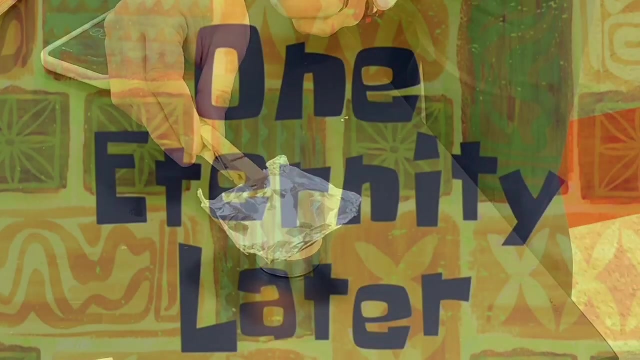 because that's when it just started to melt And we're going to put under sugar 45 seconds, All right. moving on to salt, Set my timer, Put it on there, Light my tea light, All right, And start All right. So I've been waiting here about five or so minutes.